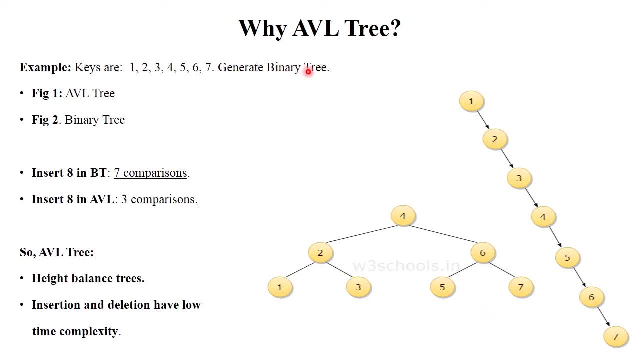 binary tree right. The concept of binary tree is the value greater than root is always on right side and value less than root is always on left side. Okay, so you generate binary tree through this numbers. then this type of tree is generated, right. 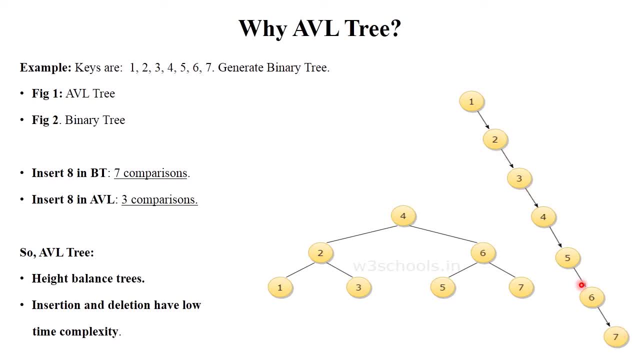 1,, 2, up to 7.. Okay, which is called right skewed binary tree Here. suppose you used AVL tree for this purpose. then this kind of binary trees or AVL trees generated. Okay, suppose you need to insert 8 in binary tree. Okay, so 8 is here after 7, right, So how? 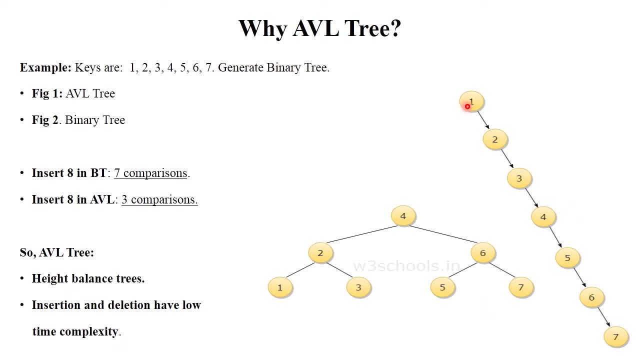 much comparisons are required. You first compare 8 with 1.. Okay, so 8 is greater than 1, then you need to compare with 2.. Again, up to 7.. Okay, so there are total 7 comparisons are required for inserting 8. 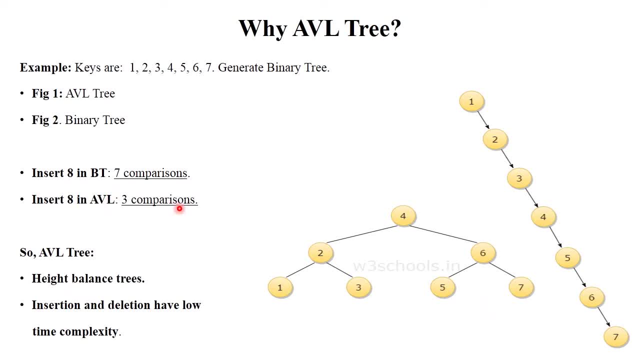 in binary tree. Okay, suppose if you insert 8 in AVL tree, so you need only 3 comparisons. You first compare with 4, then compare with 6 and then compare with 7 and insert: 8 is here. Okay, so you required only 3 comparisons and that's the reason we used AVL tree- AVL. 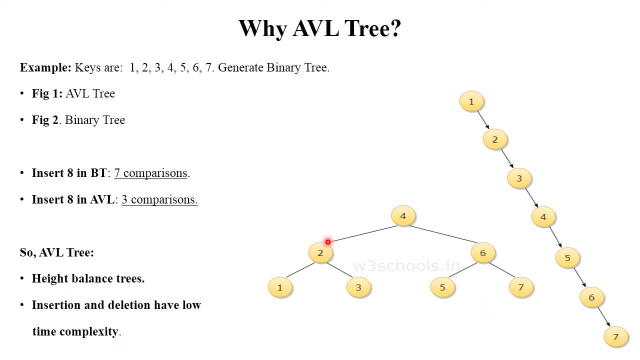 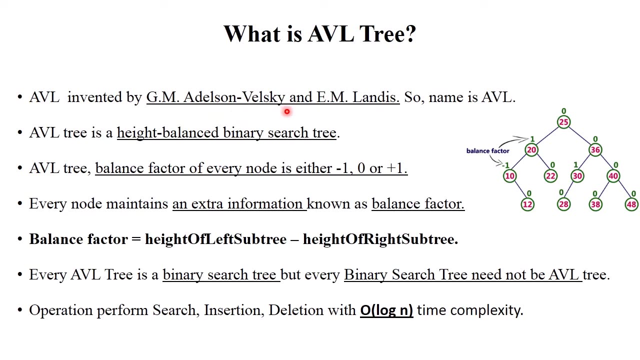 tree is a height balanced binary tree, Okay, and for insertion, deletion and searching operation It required low time complexity. Okay, so this is the reason of AVL tree. Now, what is AVL tree? AVL tree is invented by Adelson, Valesky and Landis, these three scientists. 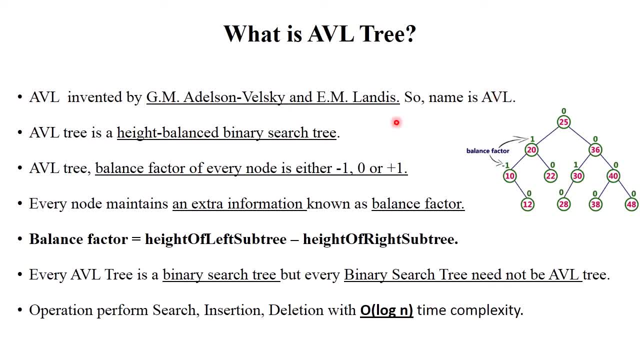 Okay, so name is AVL. Okay, AVL tree is a height balanced binary search tree, and AVL tree used one term, which is called balance factor, and balance factor of AVL tree is either minus 1 or 0 or minus 1.. Okay, so this is the height balanced binary tree and AVL tree. 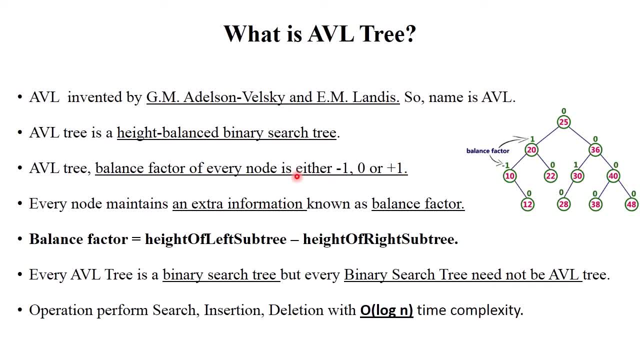 is a height balanced binary search tree and AVL tree used one term which is called balance factor of AVL tree. So the2 calculations we gotta use here is easily simple. Well, here ti will be the same problem as showing here. So the second complication which we should do will be Governance factor function. 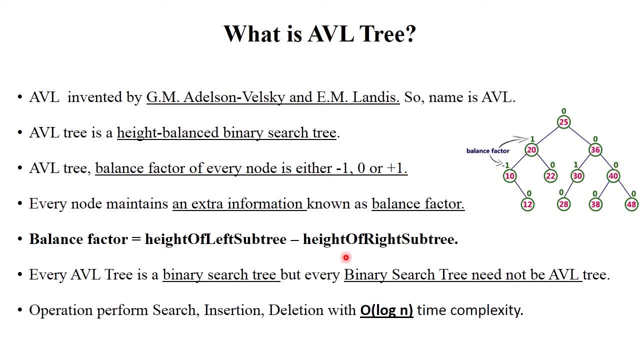 No. then tell them the second complication that you used positive valid factor: criticize 15 points, Okayӓ. So let's have another case. should create this function. 市 has remaining weit. there is only one right child, okay. so 0 minus 1 means minus 1. so minus 1 is balance factor of 10. 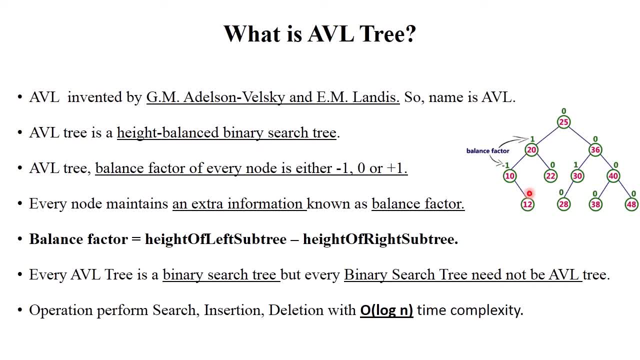 okay, so this is in this way we calculate the balance factor. so each and every tree in binary search tree, okay, but every binary search tree need not avial tree, because avial tree used property of binary search tree. so each and every operation like search, insertion, deletion. 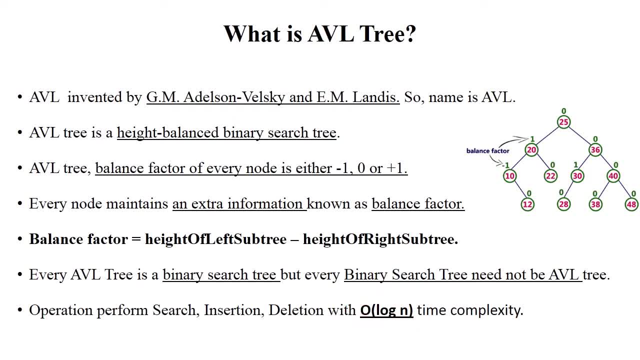 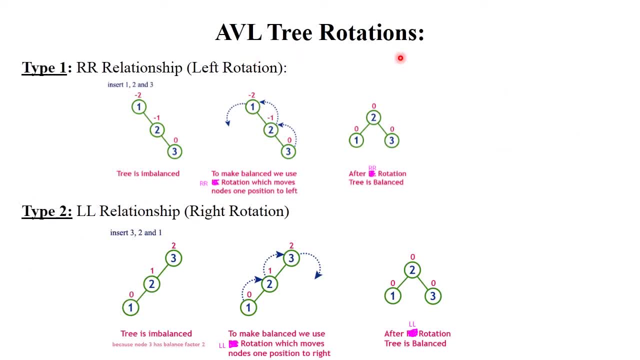 it required a big O log and time complexity in avial tree. so before try to solve the examples of avial tree, the main term is avial tree rotation. in my previous video we learn about rotation, but in red, black binary tree which perform the rotation according the colors, either red or black. but in this video avial tree perform. 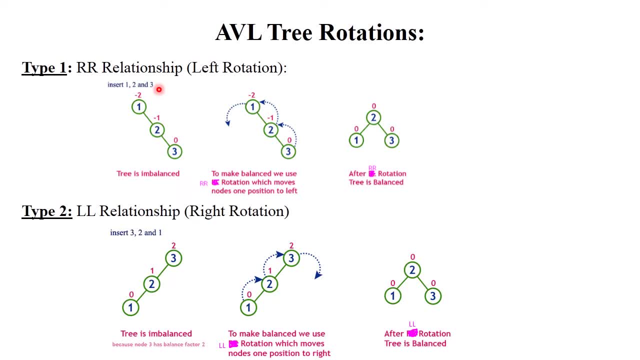 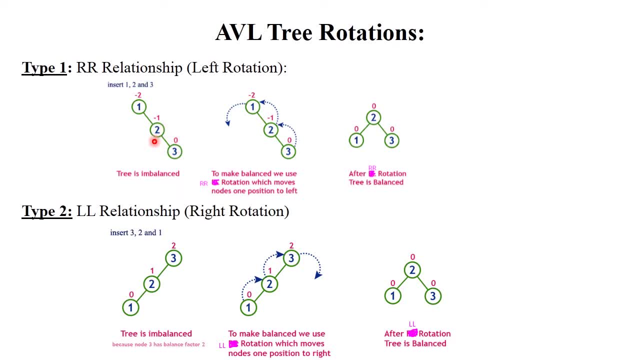 the balance factor of 3 is 0. balance factor of 2 is minus 1, that is 0, and 1, that is minus 1. okay, balance factor of 1 is left side 0 and right side 2, that is 0 minus 2 is minus. 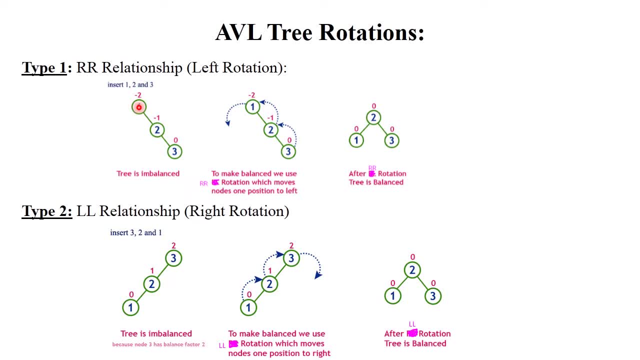 2. okay, so minus 2 is not eligible for balance factor. okay, so tree is imbalanced, clear. so when tree is imbalanced, you need to perform suitable rotation. so which rotation you perform first check the relationship here. R? R relationship, see 2 is right of 1 and 3 is right of 2- means right, right relationship. so when right right, 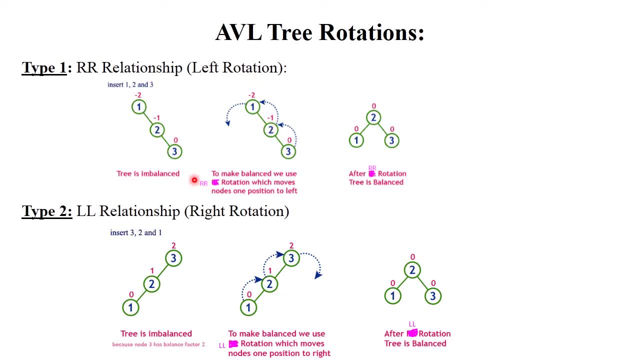 relationship occur, you need to perform left rotation. okay, so there are three nodes. okay, so performing left rotation, the middle node always become the root node. okay, so see in here this is left side. so 1 move to left, rotate rotated. 2 goes to here and 3 goes to. 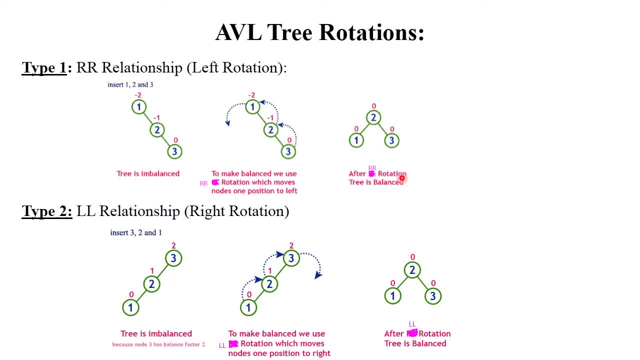 here and this tree is generated clear. so this is called left rotation. you perform left rotation here. now again check balance value. the balance factor of 1 is 0 because no left right sub tree. balance factor of 3 is 0 and balance factor of 2 is also 0: 1, 1 1 minus 1 equal. 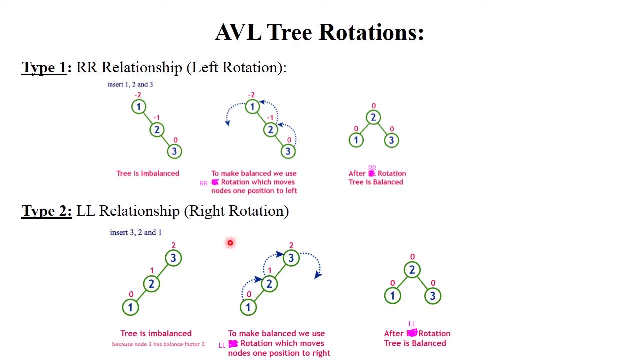 to 0. okay, so similar concept applied in other video, other rotations: okay. so see, this is LL relationship. LL relationship perform always right rotation. in this example, balance factor of 3 is 2. okay, because left side 2, right side 0, 2 minus 0. 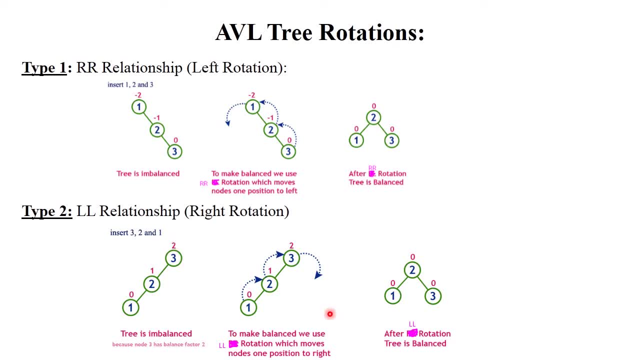 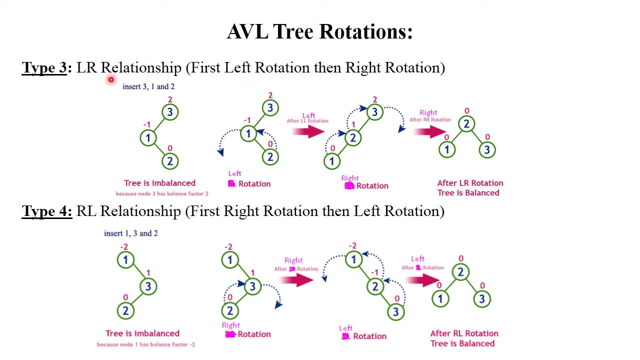 2. okay. so this tree is imbalanced. you need to perform right rotation here, so middle node become root. now 3 and 1. this is called right rotation. okay. so next rotation is left rotation and right rotation. okay, if LR relationship occur, see in this example. 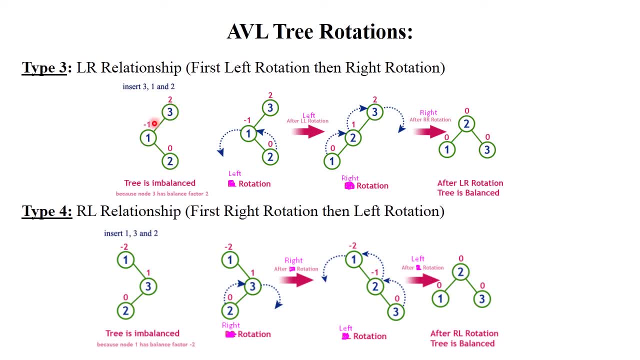 3, 1 and 2. okay, the balance factor of 3 is 2 because because it is minus 1, right and it is 0. so balance factor of 3 is become 2, so it left and right. okay, so there is LR relationship occur when. 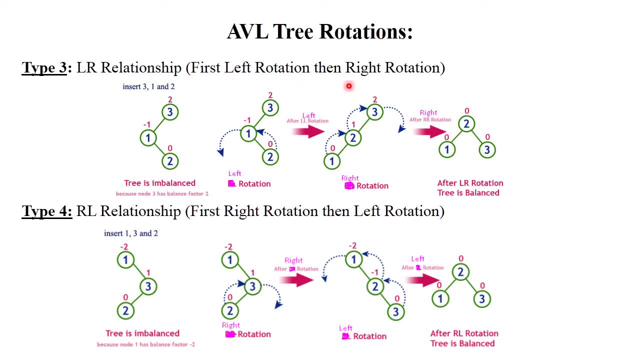 LR relationship occur, you need to first perform left rotation, after that you need to perform right rotation. so first rotation always will perform on the two nodes and right rotation can be performed on three nodes. see here. first you need to perform left rotation. okay, see here. so left rotation means one goes to here on left side and two goes to on. 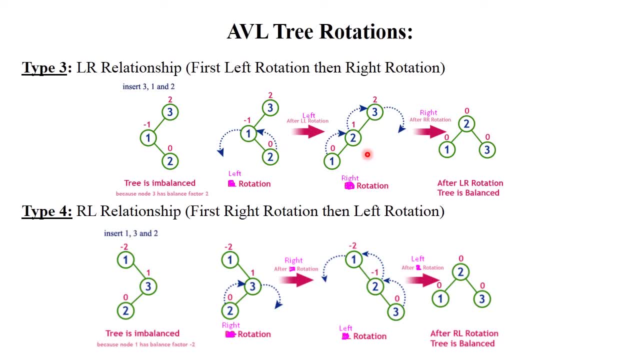 the place of one. so now this tree is generated, now you need to perform right rotation on three nodes. so perform right rotation on this left rotation generated tree. three goes here, two become root node and one become their left node. always remember when you perform operations on three nodes, okay, so 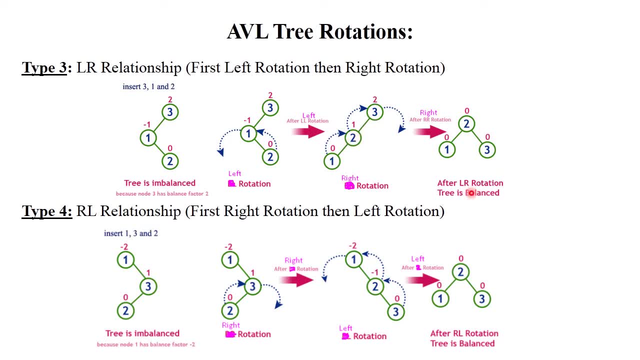 middle node always become the root. okay, so here tree is balanced. the next opposite of LR relationship is RL relationship and you need to perform first rotation and then left rotation. RL means right rotation first, then left rotation. okay, see, here there is right and left relationship. tree is: 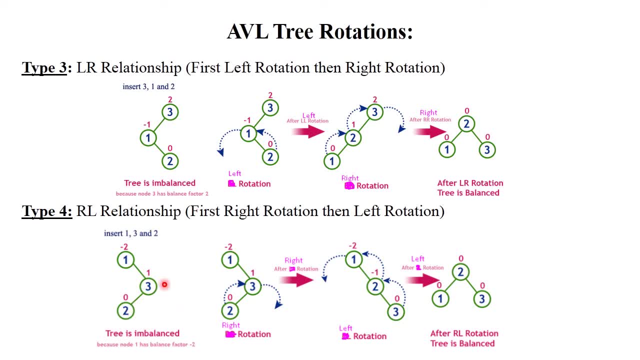 imbalanced due to balance factor. so you need to first perform right rotation here. so three goes around right side and two goes in upward direction. okay, now, after right rotation, they perform left rotation. okay, so from this three node, middle node, become the root node. okay, and perform left rotation, move it on left side, okay. 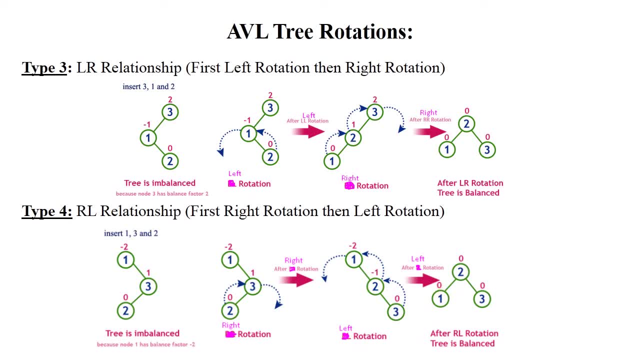 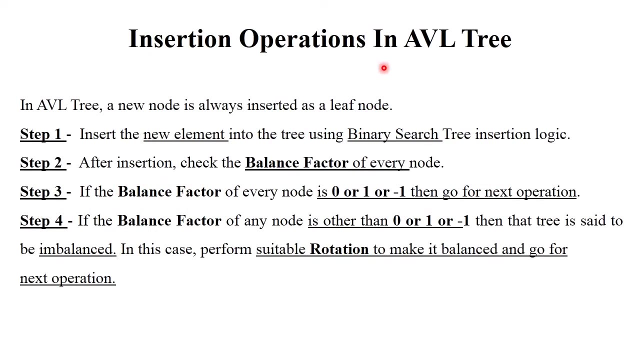 now tree is balanced. so this is all about AVLT rotation. you need to use this rotation while trying to solve the examples. see, now we learned about how to solve the examples of AVLT. so first, insertion operation in AVLT. the first step is you need to insert element according to binary search tree logic. okay, 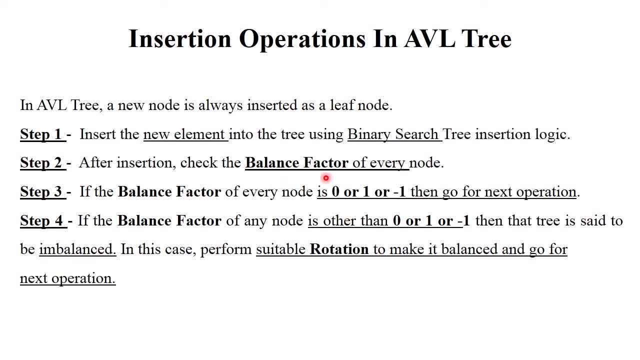 second step: after insertion, you need to check balance factor of each and every node. third step: if balance factor of every node is zero, one or minus one, then go for next operation, okay. and if balance factor of any node is other than 0, 1 or minus 1, then tree is imbalanced or at that time you need to perform suitable. 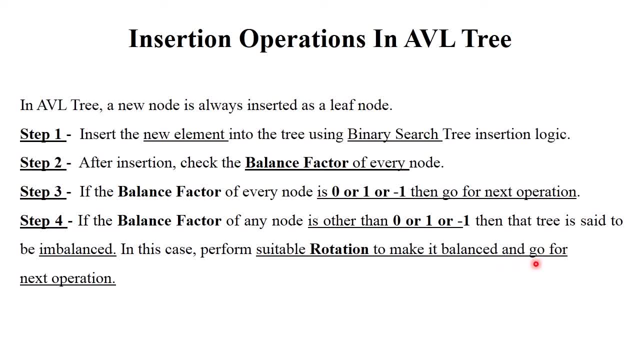 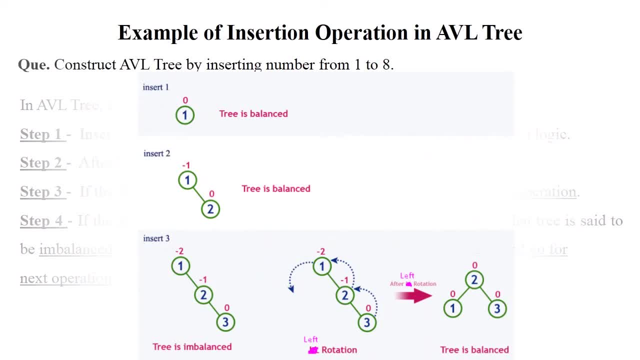 rotation and make the trees balance, okay, and then go for next operation. so let's see how insertion operation is performed on avial tree. okay, so given operation is construct avial tree. okay, by inserting number from 1 to 8. okay, so see, here you need to add or insert numerical values. 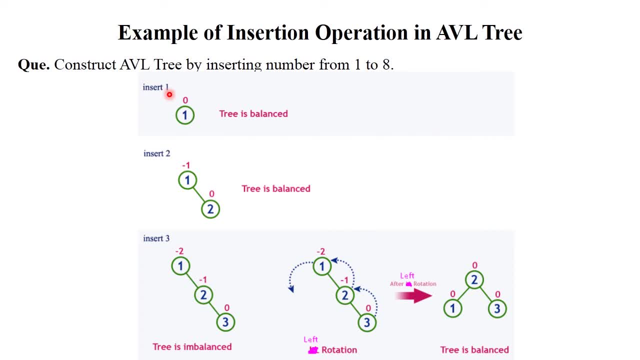 as per the sequence. okay, so first insert 1. tree is empty. you need to insert 1 and trees balance. because there is no left and right subtree, the balance factor of 1 is 0. okay, now you need to insert 2. according the binary search tree logic, 2 is greater than word. now 2 is move to right side. 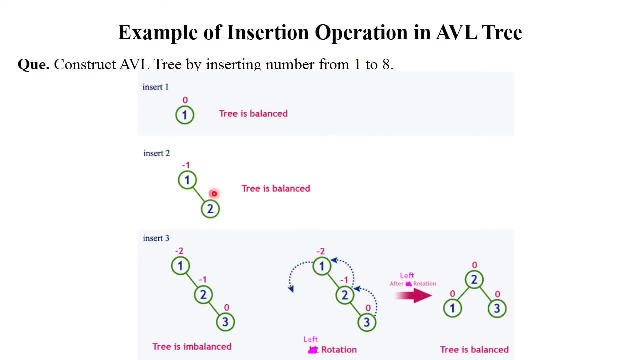 okay, then again calculate balance factor. balance factor of 2 is 0 and balance factor of 1 is minus 1, because left subtree 0, right subtree 1, 0 minus 1 minus 1. okay, now tree is balanced. so again now insert 3. 3 is greater than 1, 3 is greater than 2 and 3. 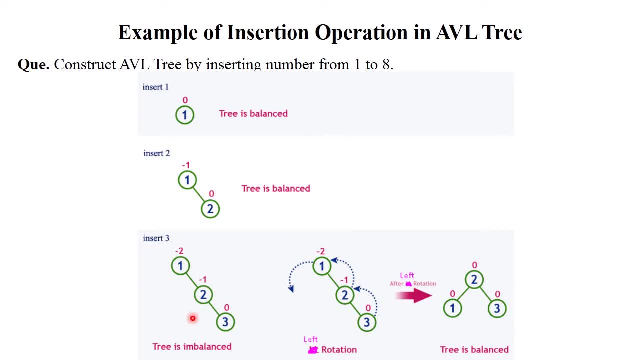 placed here. okay, now again calculate balance factor. the balance factor of 3 is 0, okay, 2 is minus 1 and 1 is minus 2. okay, so trees. now tree is imbalanced because one balance factor of 1 is minus 2, because left subtree 0 and right subtree 2, there are two edges, okay. so 0 minus 2 minus 2. 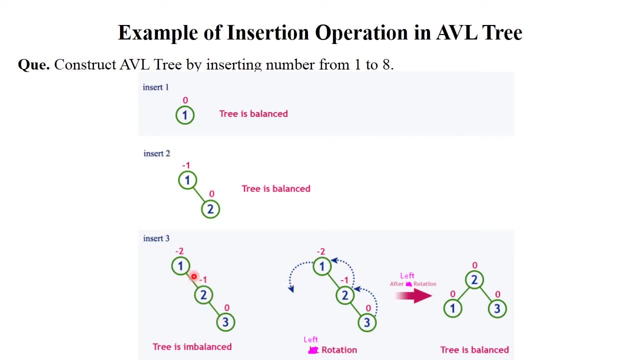 so there is rr relationship. okay. so when rr relationship occur, you need to perform left rotation. okay. there are total three nodes. the middle node become the root, okay, and perform left rotation. so one move on left side, 2 becomes root and 3 on right side. clear, now this tree is generated and balance. 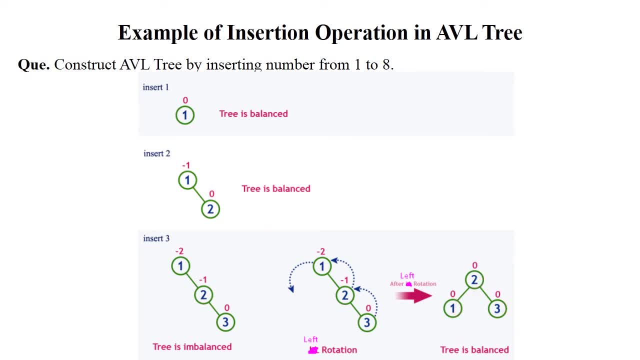 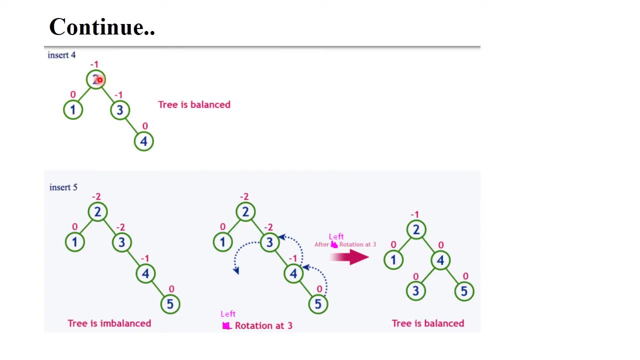 factor of 1, 2, 3 is 0 and now tree is balanced clear. now you need to insert 4. okay, so 4 is greater than 2, 4 is greater than 3, 4 placed here. now calculate balance factor. balance factor of. 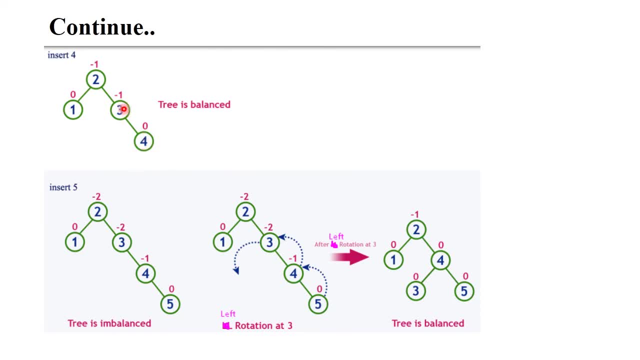 4 is 0 because no left and right subtree. balance factor of 3 is minus 1 because here is 0 and here is only 1. that is 0 minus 1 minus 1. okay. balance factor of 2: here is 0 and here is 2. 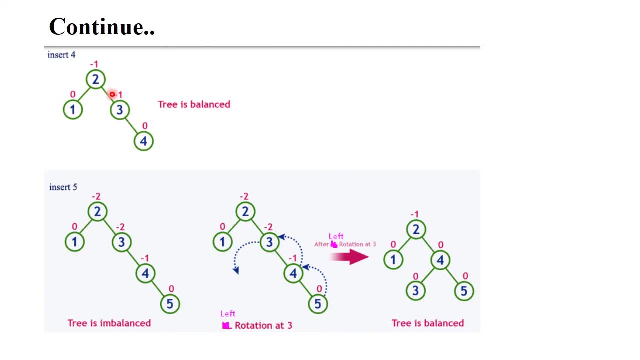 okay, 1, 2. so 0 minus 2, 0 minus 2, but here minus 1. we already calculated. okay, so where it becomes minus 1 and it becomes 0, okay, so tree is balanced. you need doesn't need to perform any rotation. 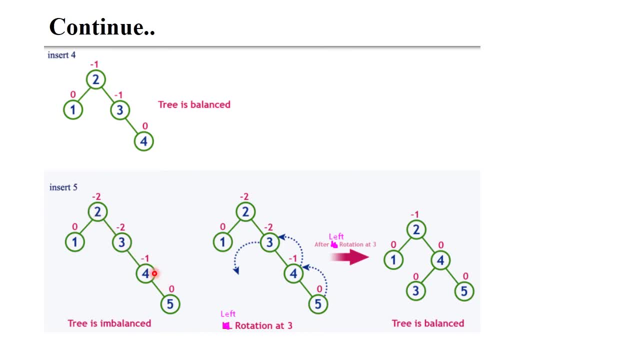 now insert 5. okay, so again you need to 5 insert after the 4 again check their balance factor. balance factor is here 0, here minus 1 and here minus 2. okay, after insertion you need to calculate balance factor. so balance factor of 3 is minus 2. okay, so it now need you need to. 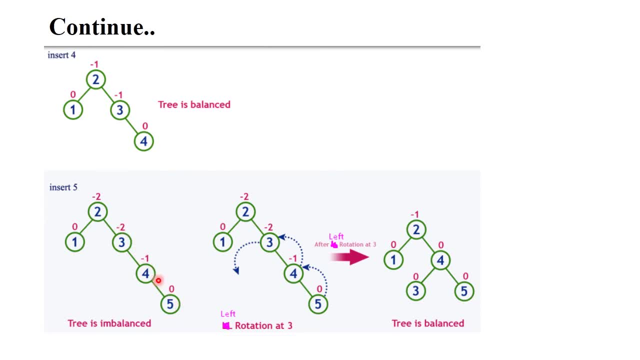 perform rotation here. so it is rr relationship- okay. so when rr relationship occur, you need to perform left rotation. so rotation perform on this. 3 nodes- okay. middle node become the root. now 3 goes to left side, 4 becomes the root. so here 8 returns to 12 and here 6 returns to 15. fine bushy. 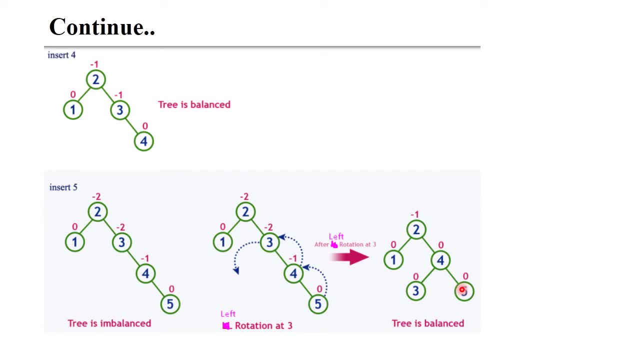 and here 2 returns to 12. so Meat I am beginning to do with a J, others after insertion, here noch a and phi u is on right side of 4. Clear, Okay. So now again check their balance factor. The balance factor of tree is 0, 0, 0 and here 0 and minus 1.. Okay, Means tree is balanced, Clear. 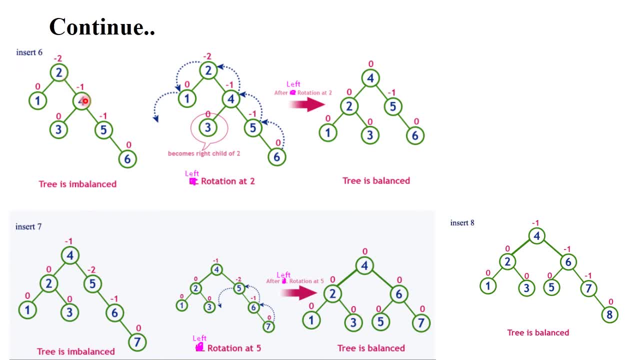 Need to insert 6.. Okay, 6 greater than 2, greater than 4, greater than phi u, and you need to 6 placed after the phi u. Okay, So check their balance factor. The balance factor of 2 is minus. 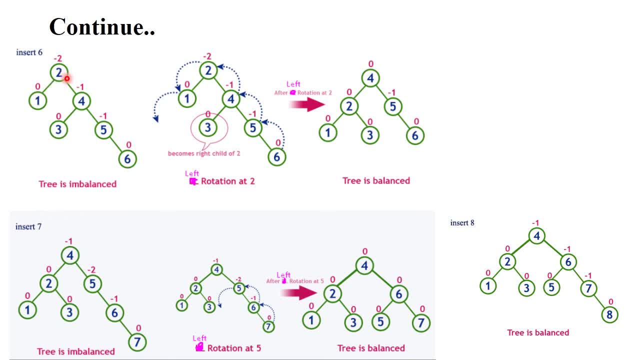 2.. Okay, See, here is 1, and right tree is 1, 2 and 3.. Okay, So 1 minus 3 is minus 2.. Clear, So which relationship occur here? Tree is imbalanced. Okay, So there is R-R relationship. 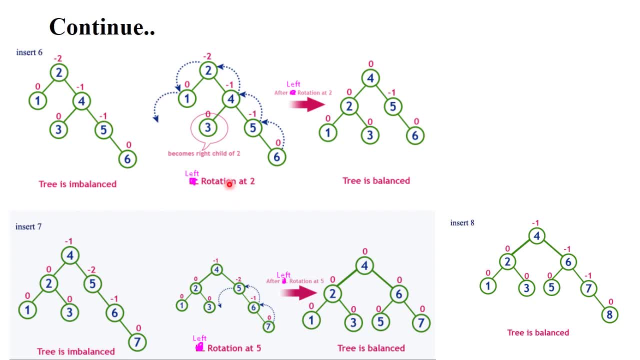 Okay, So when R-R relationship occur, you need to perform left rotation, See here. So rotation perform on this 3 nodes. Okay So middle value is 4.. 4 is become root, 2 is goes to left side. 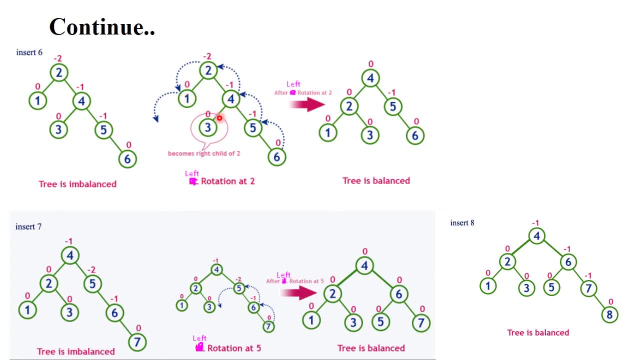 and 1 again goes to left side. Okay, And this 3 is becomes the right child of this 2.. See, in this example, 4 becomes root and 3 becomes right child of 2.. After left rotation, this 3 is generated and now this tree is balanced. 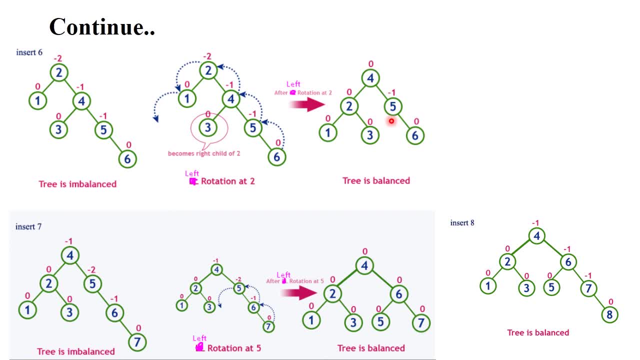 because balance factor is 0,, 1 and minus 1.. Clear, Now you need to insert 7.. So 7 insert is here according the binary search tree logic. So again, check the balance factor. but balance factor of phi u. 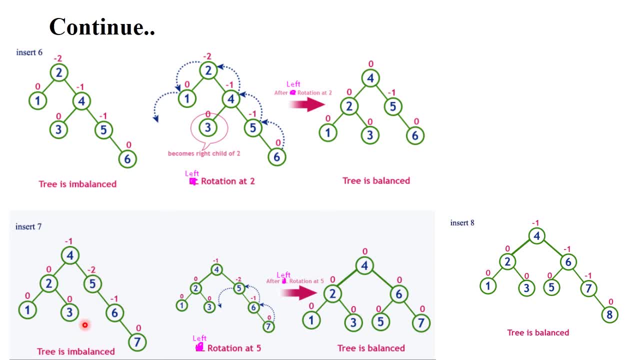 is minus 2.. See, here is 0 on left side and right side, 2.. 0 minus 2 minus 2.. Okay, Then which relationship occur? Right-right relationship. When right-right relationship occur, you need to perform left rotation. Okay, So left rotation perform on this 3 node. The middle node becomes. 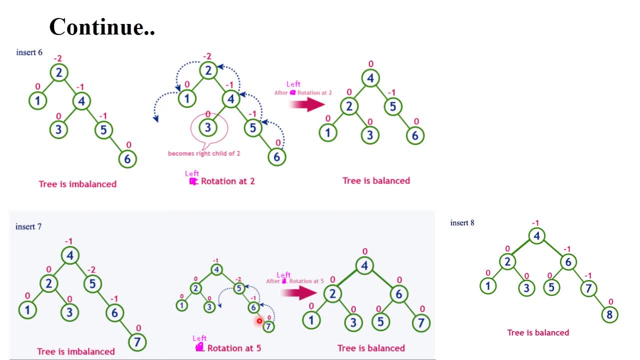 root. Okay, So phi u moves on left side, 6 moves to on the place of phi u and 7 move to 6.. Okay, Now this tree is generated: 6., 5,, 7.. Then again check balance. factor. Tree is balanced And at last you need to insert 8. You. 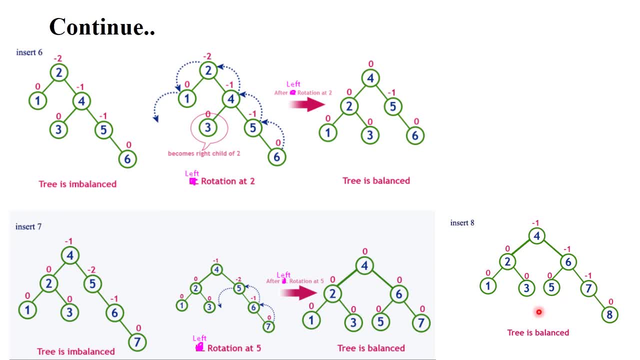 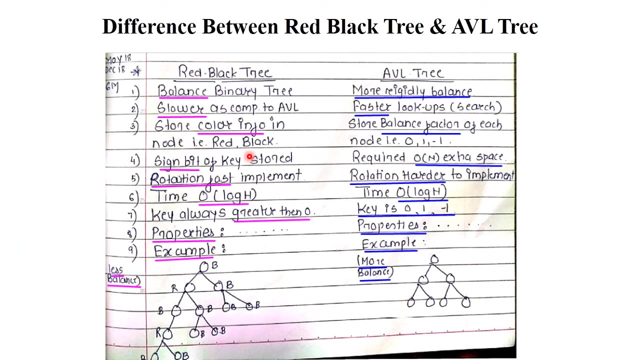 insert 8. here Again, check the balance factor of each and every node. Okay, Now tree is balanced. Clear, Hope. so you understand this example and you need to practice more and more examples. So your concept is clear. Okay, Difference between red-black tree and avial tree. So red-black tree. 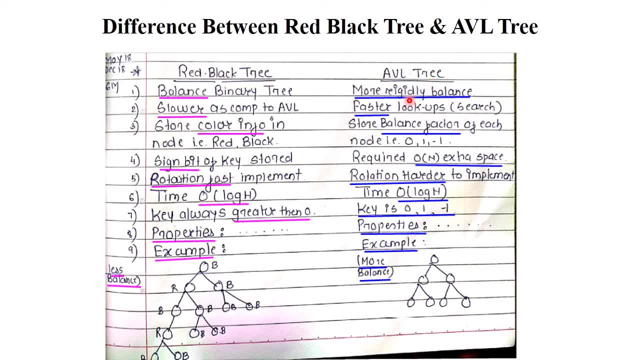 is balanced binary tree, Okay, But avial tree is balanced binary tree. So red-black tree is balanced binary tree. Okay, But avial tree is balanced binary tree. So red-black tree is balanced binary tree. So avial tree is more balanced than red-black tree. In red-black tree perform the searching operation is slower as compared to avial tree. 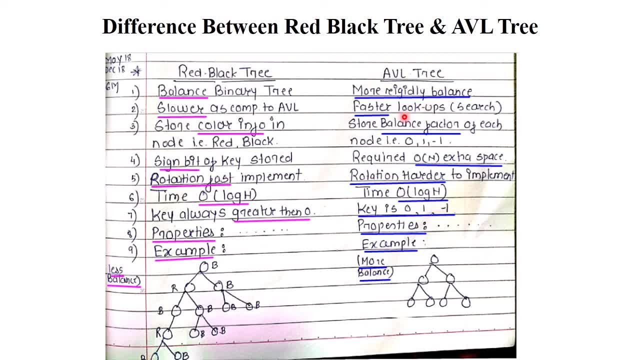 Avial tree perform fastly lookup or search operation. Okay. Red-black tree store color information of node and avial tree store balanced factors like 0,, 1 and minus 1.. Clear Red-black tree rotation is very fast as compared to avial tree. Okay, So time. complexity of both red-black tree and avial tree is 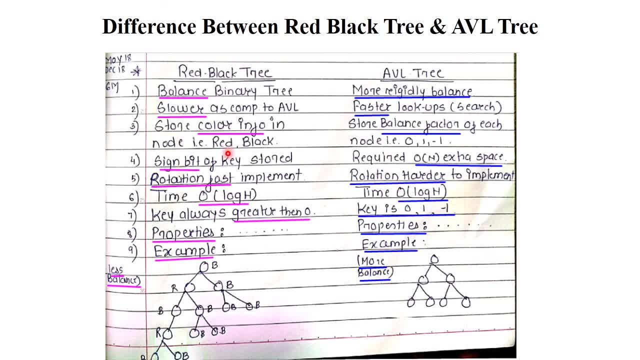 big or Long and But there is difference between the space complexity. it requires sign bit of key stored and require bigger and Extra space for storing this numerical value or balance factor. Okay, In red black tree keys always greater than zero. okay, But avial tree is 0, 1 and minus 4.. Okay, So we learned about. 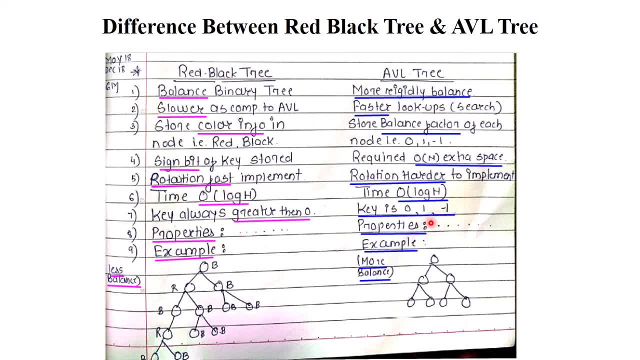 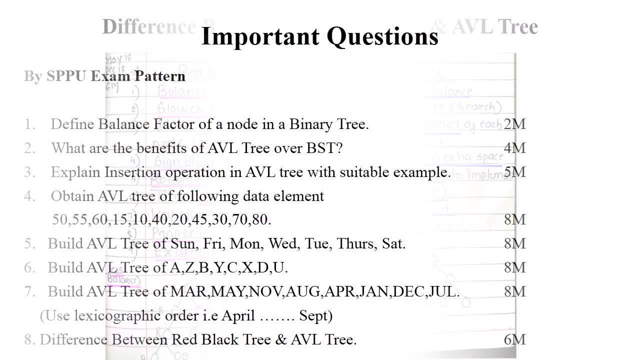 properties of red-black tree. in my previous video And now in previous slide, we learn about properties of avial tree. Ok, so see this example: Rail black tree is less balanced than avial tree And avial tree is more balanced Clear. Here are some important questions which mostly asked in SPPU exam pattern. 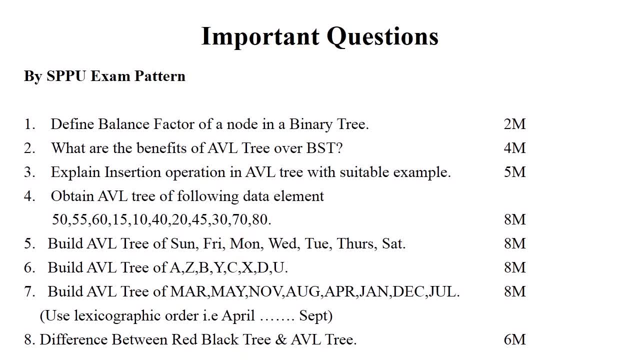 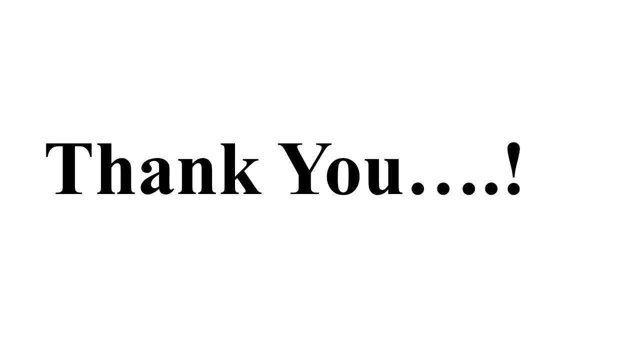 Try to solve these examples and keep practicing, Thank you. This is all about avial tree, Properties of avial tree And insertion operation in avial tree And avial rotation. So keep practicing it, Thank you.